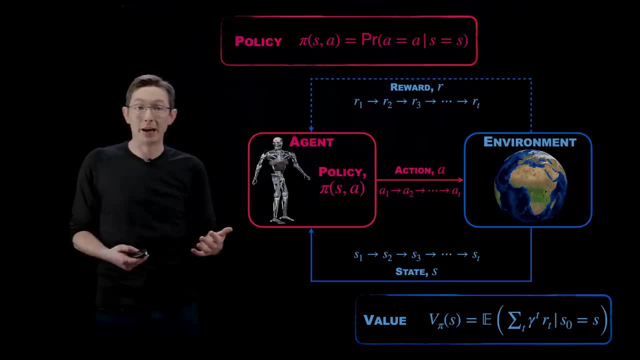 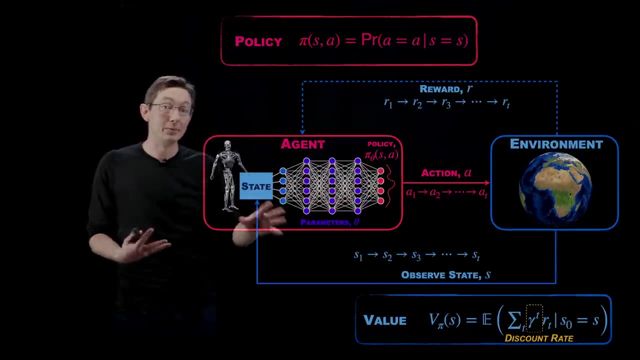 to augment this picture by introducing deep neural networks, for example, to represent the policy. So here we have, now we've replaced our policy with a deep neural network. So this pi is parameterized by theta, where theta describes this neural network And again it maps the current. 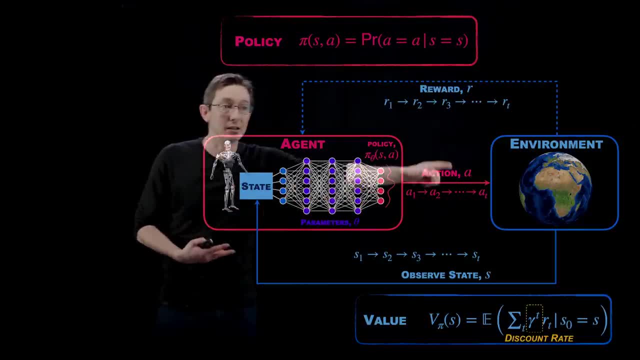 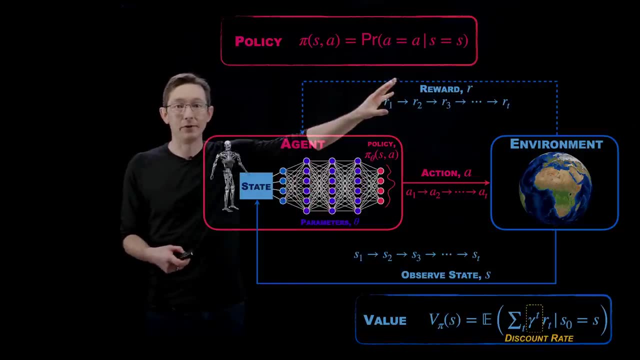 state to the best probabilistic action to take in that environment, And so the whole name of the game is to update this policy to maximize future rewards. And again we have this discount rate gamma here that says that rewards in the nearer future are worth more than rewards in the distant. 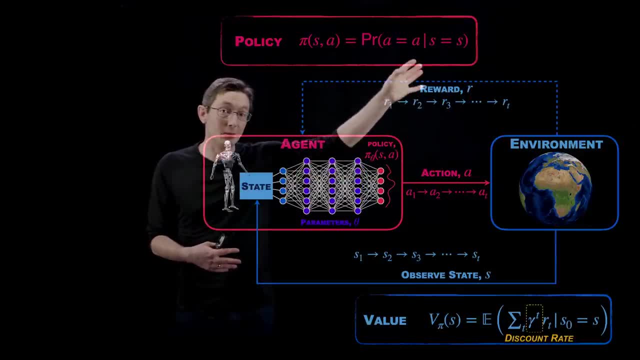 future. Okay, Because, again remember, these rewards are going to be relatively sparse and infrequent most of the time, because we're in a semi-supervised learning framework where these rewards are only occasional And so it's difficult to figure out what actions actually. 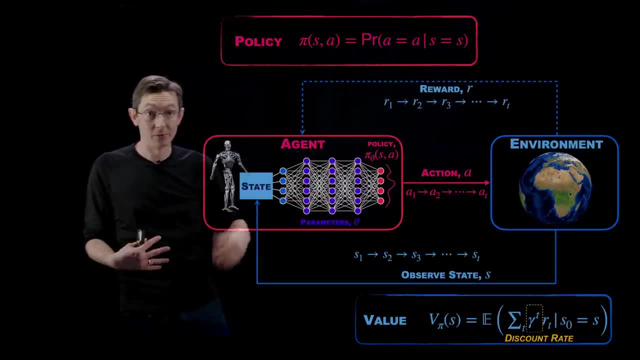 gave rise to those rewards. This is going to be a pretty hard optimization problem to learn this best policy of what actions to take. But you know, and actually the whole reinforcement learning paradigm is biologically inspired. It's essentially inspired by this observation. So 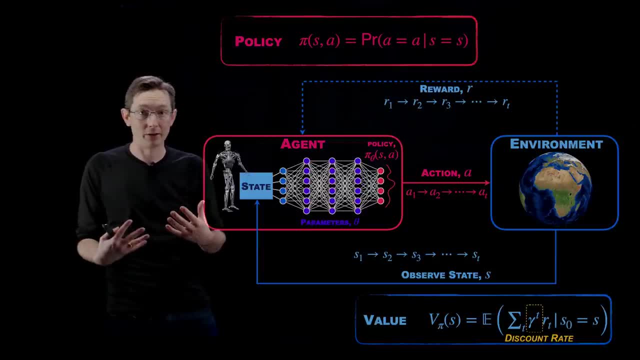 there's this notion called Hebbian learning. You might have heard this before And the little rhyme it goes: neurons that fire together wire together, And basically what that means is that when you have neural activity, kind of when things fire together, they will essentially strengthen the 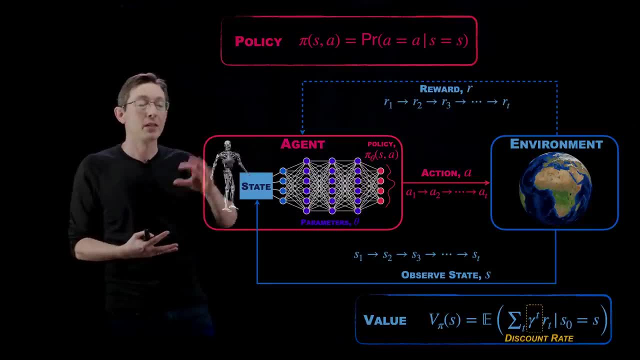 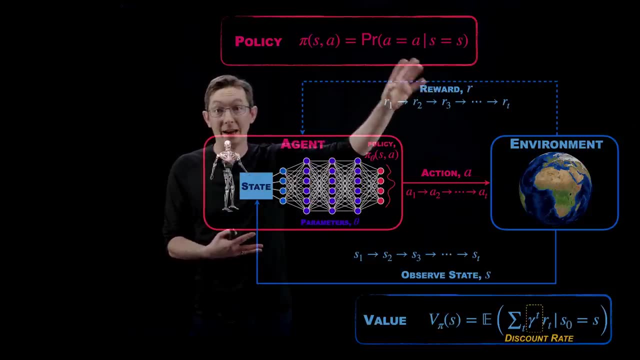 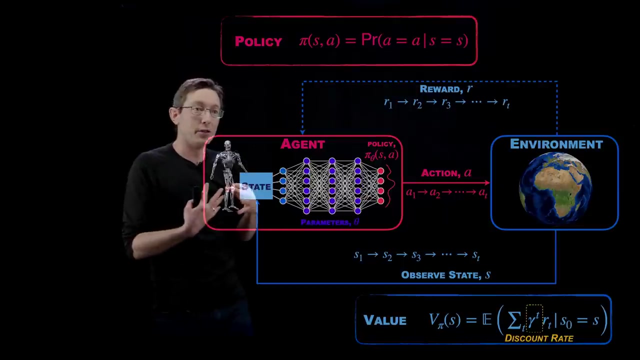 wiring and the connections between those neurons in biological systems, And so in these kind of deep reinforcement learning architectures, the idea is that the reward signal that you get occasionally should somehow strengthen connections that led to a good policy, when, when the right policy is firing, when these neurons are connected in a way that causes the policy. 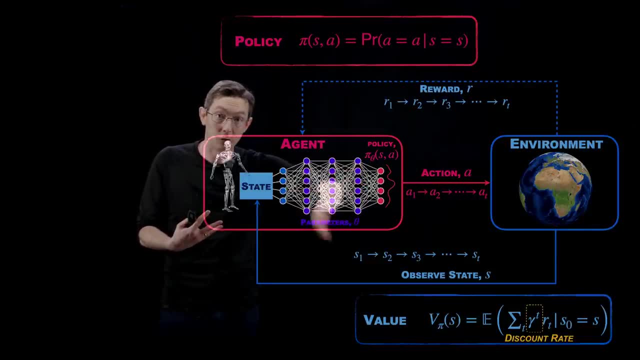 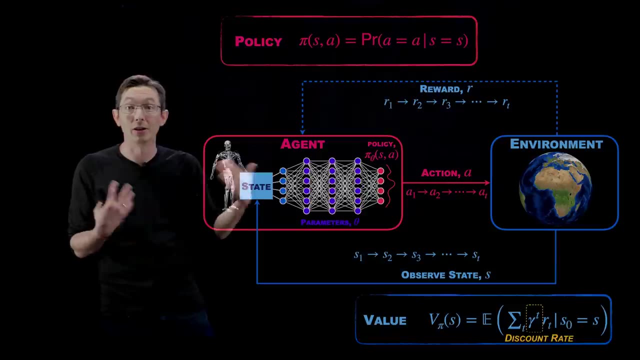 the correct policy and you get a reward. you want to somehow reinforce that architecture And there's lots of ways of doing this, you know, essentially through back propagation and so on and so forth. So another area where a lot of research is going into deep learning. 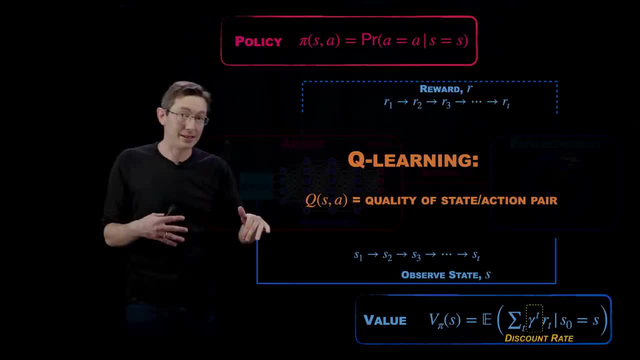 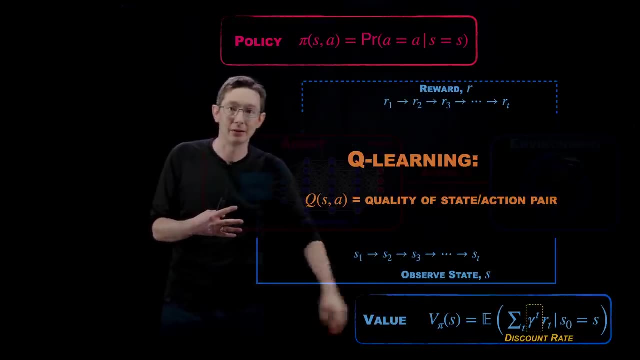 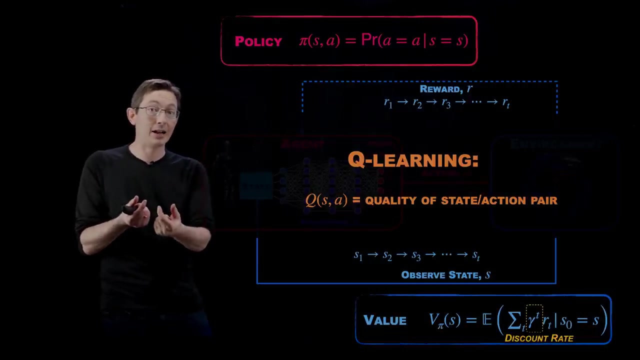 for reinforcement learning is called Q-learning- I talked about this in the last video- where this Q or quality function essentially kind of combines the policy and the value and it tells you jointly how good is a current state given a current action? A, okay, And so assuming that I do the best, 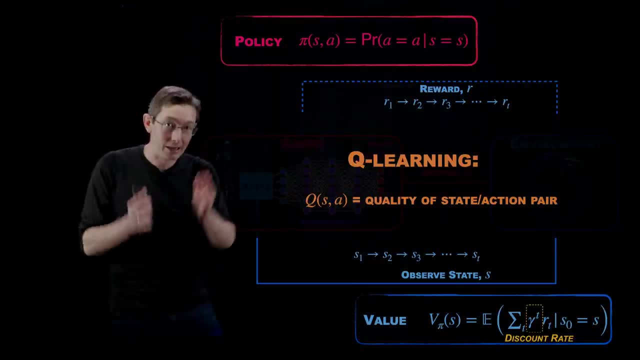 possible thing for all future states and actions. So right now, if I find myself in state S and action A, I can assign a quality based on the future value that I expect, given that state and given the best possible policy I can cook up. And so again there are deep Q networks where you learn this quality function. 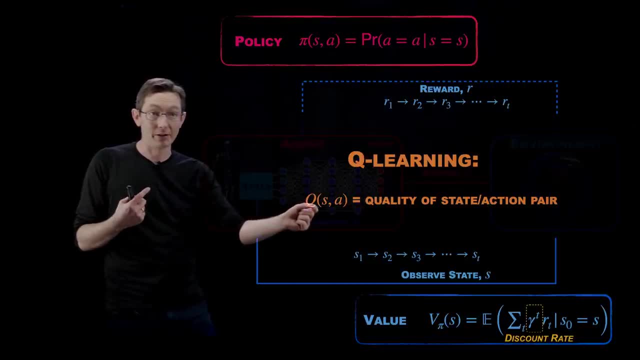 And once you learn this quality function, then when you find yourself in a state S, you just look up the best possible A that gives you the highest quality for that state, And this makes a lot of sense. This is a lot like how a person would learn how to play chess. 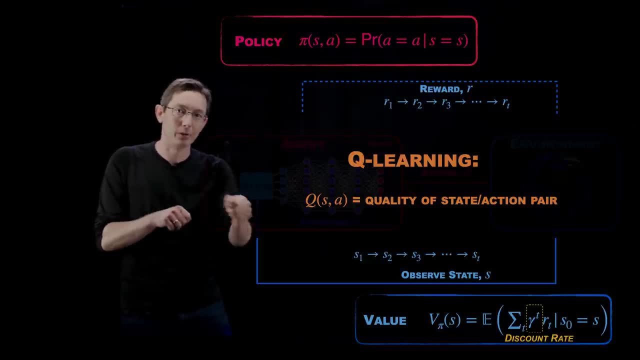 is, they would kind of simultaneously be building a policy of: okay, here's how I move in these situations, These are the trades I'm willing to make, And you're also building a value function of how you value different board positions and kind of. 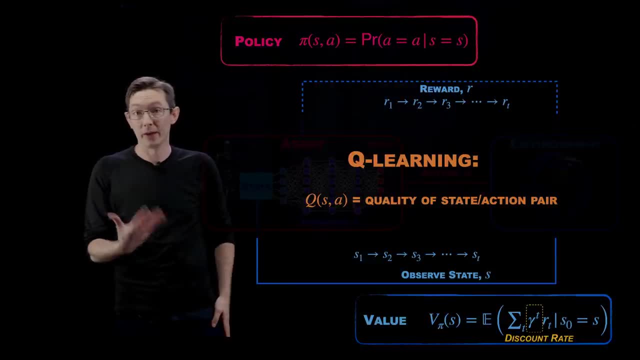 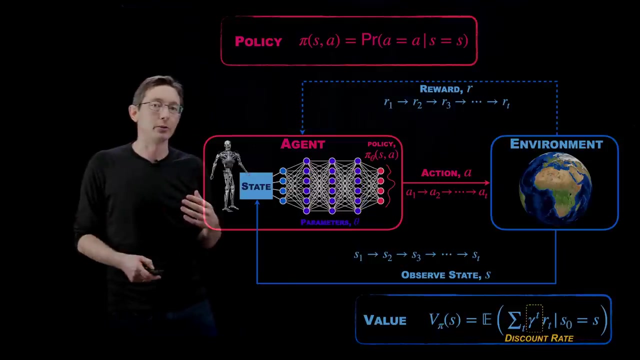 how you gauge your strength and the strength of your position, based on the state. So it kind of makes sense that this would be an area for really expanding with deep neural networks, because these functions might be very, very complex, functions of S and A, and that's exactly what neural networks 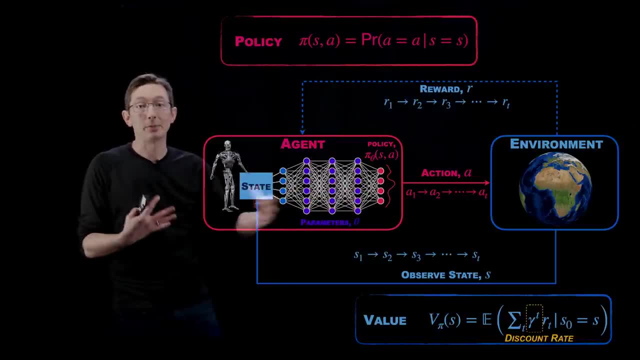 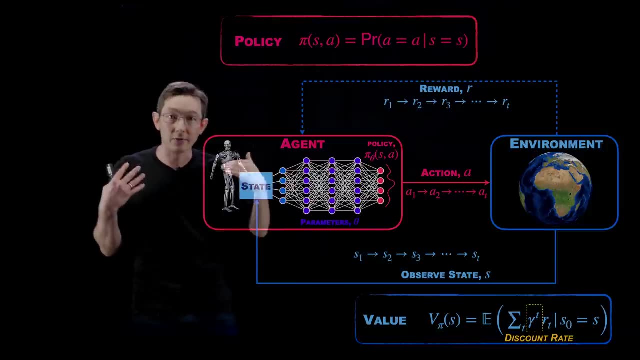 are good at is giving you very, very complex, representing very complex functions, if you have enough time to do that. So I think that's a really good idea. So that's what we're talking about here. These still suffer from all of the same challenges of 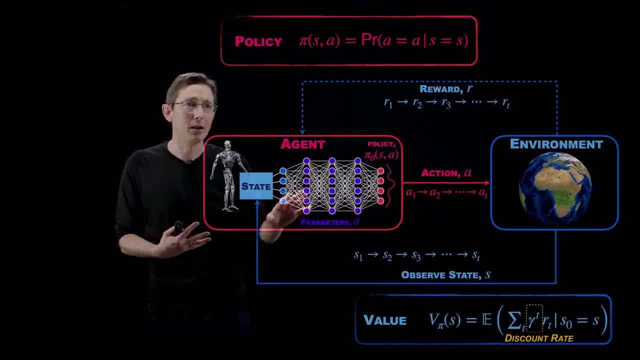 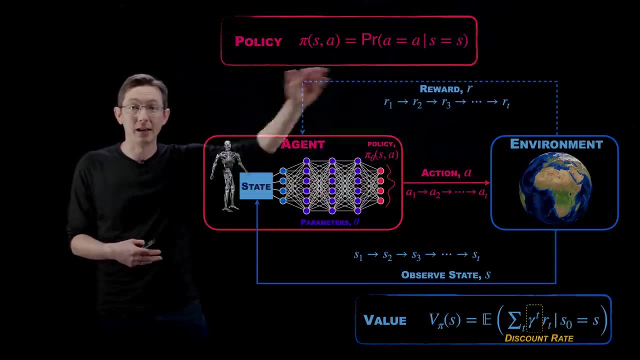 regular reinforcement learning, like the credit assignment problem. So the fact that I might only get a reward at the very end of my chess game makes it very hard to tell which actions actually gave rise to that reward, And so you're going to do some of the same things that you would normally. 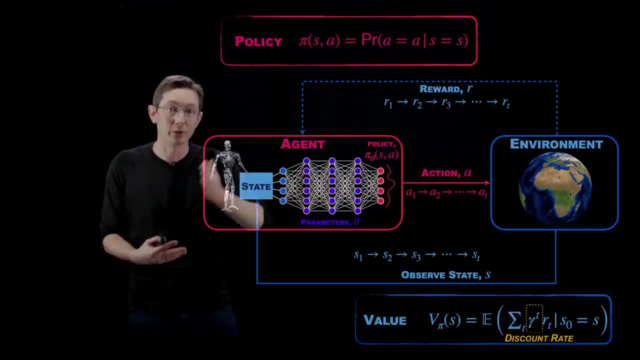 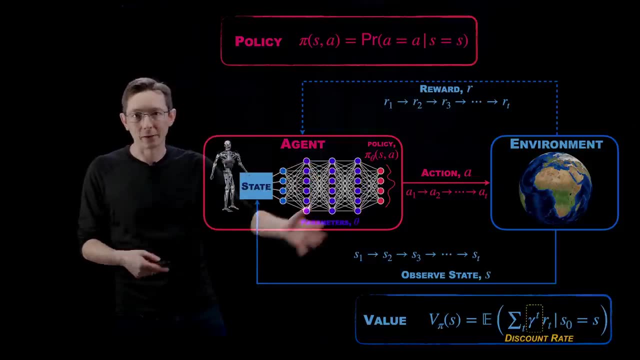 do like you might use reward shaping to give intermediate rewards based on some expert intuition or guidance, And there's lots of other strategies like hindsight, replay and things like that. okay, But the basic idea is we're going to take the same reinforcement learning architecture and we're going 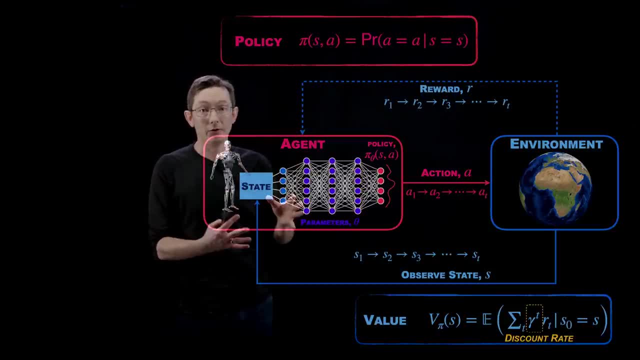 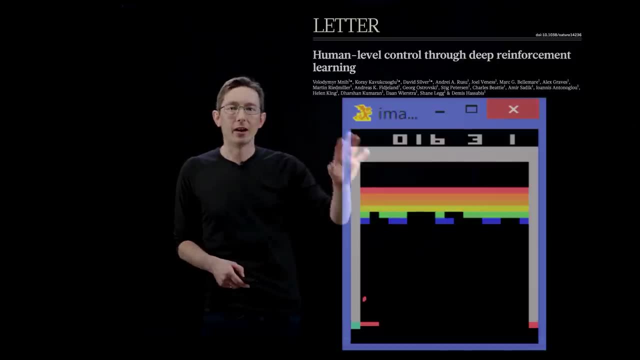 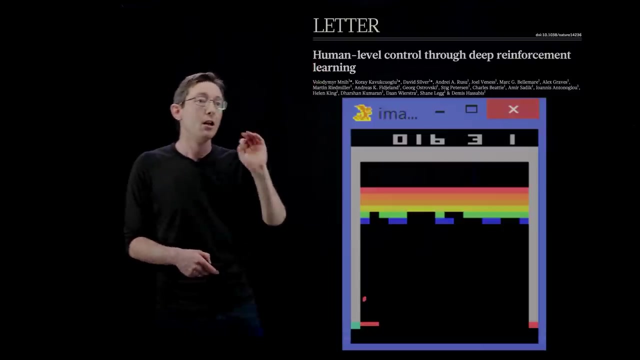 to either replace the policy or the Q function with a policy network or a Q network. Good, And all of this kind of exploded on the scene because of this 2015 Nature paper: Human-Level Control Through Deep Reinforcement Learning, where these authors from DeepMind 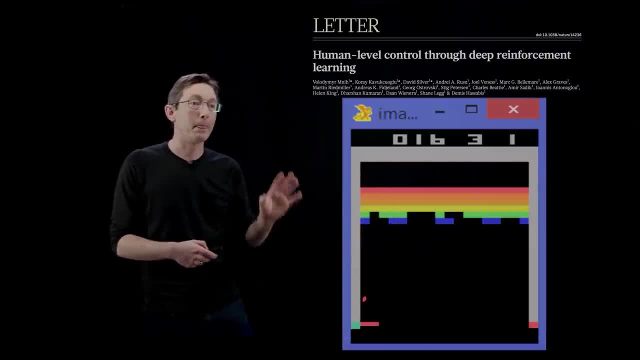 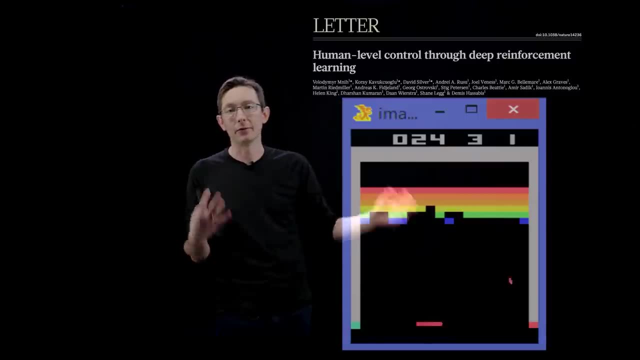 essentially showed that they could build a reinforcement learner that could beat human-level performance in lots of classic Atari video games. So I'm going to hit play. I love this one. This is one of the first ones that got me really excited about this. So this reinforcement learner is 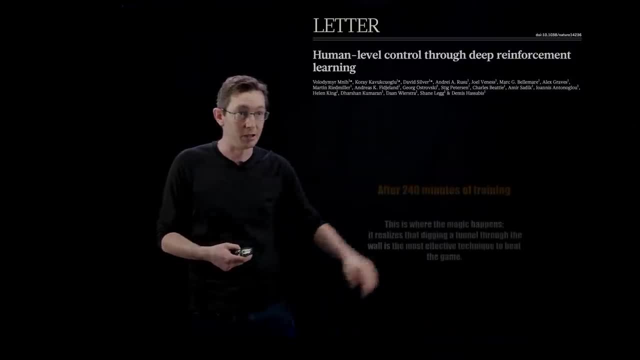 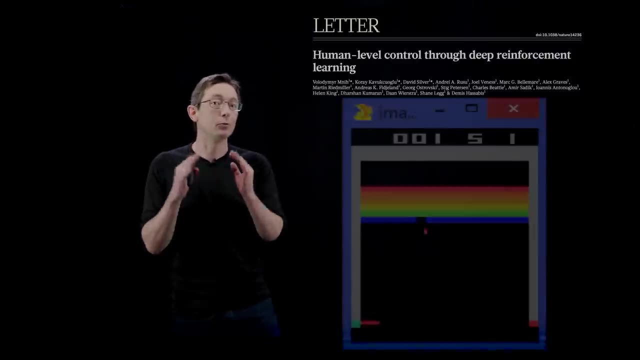 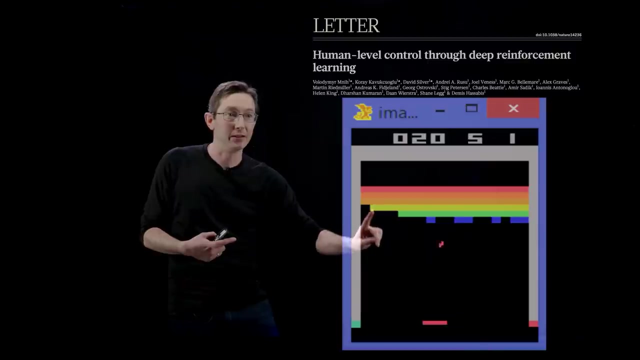 essentially trying to maximize this score by breaking all of these blocks, And after a few hours of training it has an epiphany that only really excellent human players ever reach. So it essentially finds an exploit in the game where it realizes that if it tunnels in one 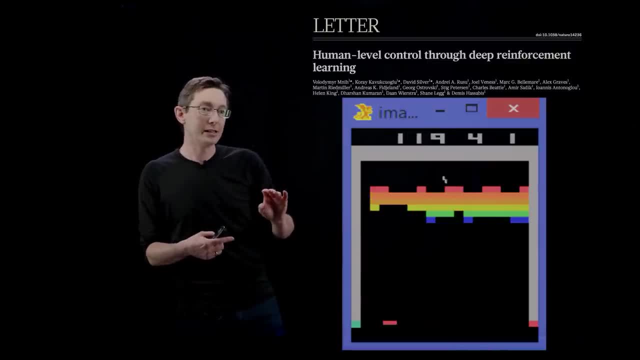 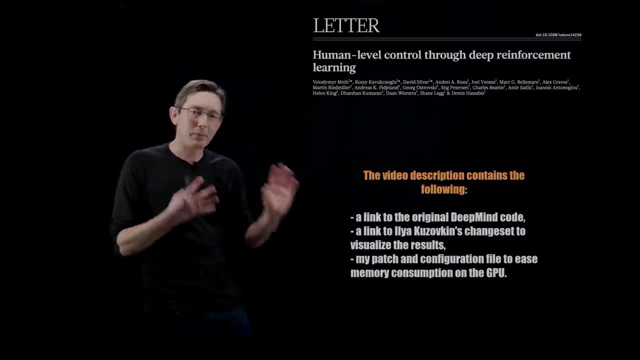 side, so it's going to tunnel through here. if it tunnels through one side, it can essentially use the physics of the game to break all of these blocks for it, And that's pretty amazing. So it, in a short amount of time, learns a really advanced strategy that only a few humans, only a small 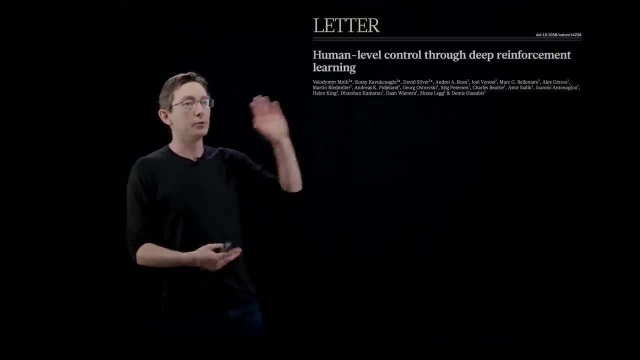 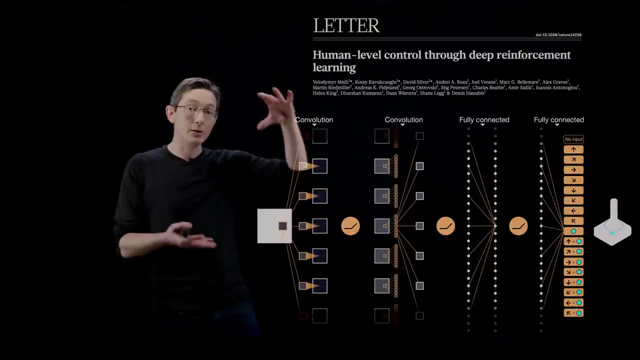 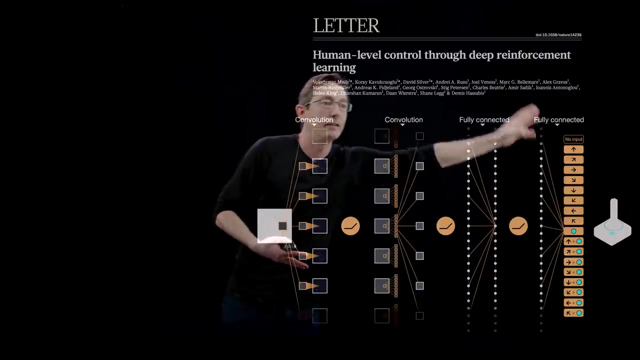 percentage of humans would actually learn eventually, So really impressive. This is a beautiful paper, by the way. You should read it. I should go read this. They talk about how they actually build their networks. So they use the pixels of the screen itself as the input and they use convolutional layers and fully connected layers. eventually, 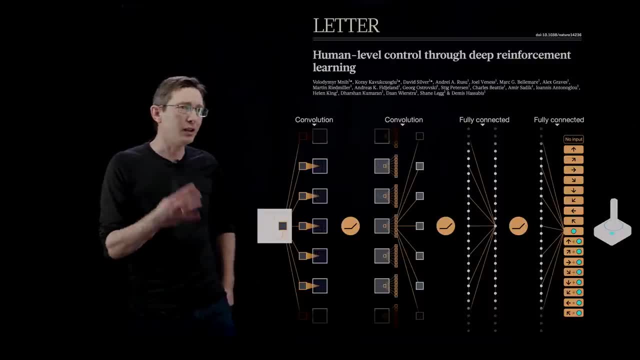 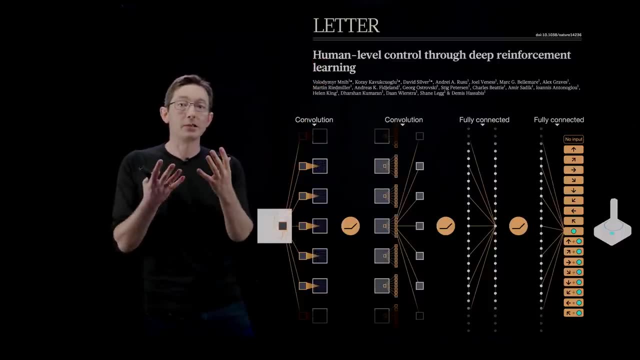 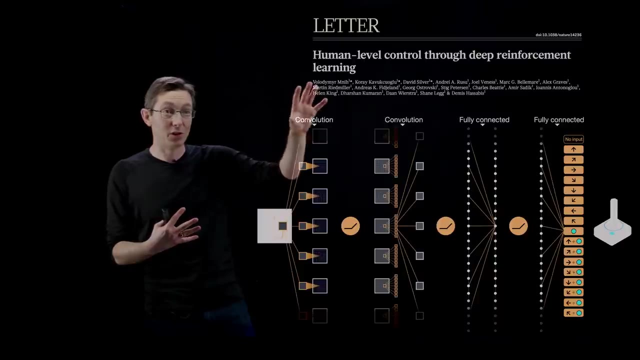 deciding what the joystick should do, what actions to take And a lot like other examples in neural networks. this was the paper that really brought reinforcement learning and deep reinforcement learning back to everyone's, to the forefront of everyone's mind, because this showed: 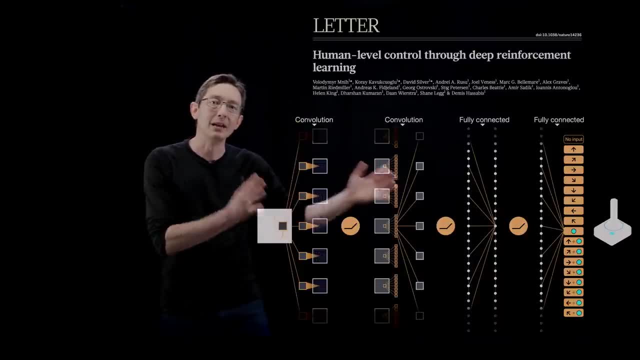 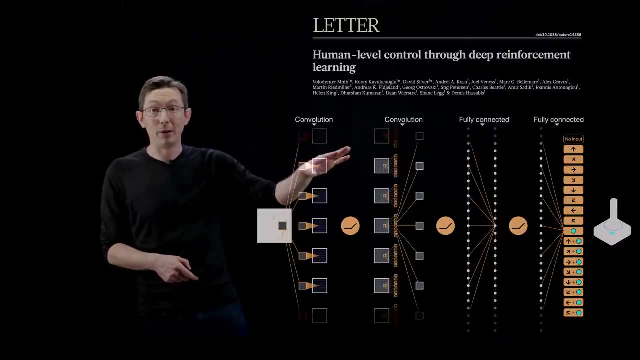 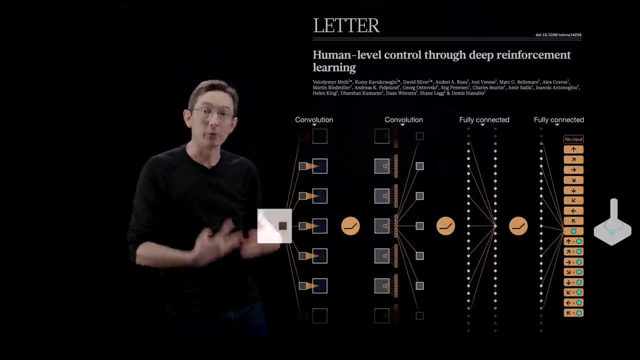 performance that hadn't been attainable before. So this is a lot like the image net of reinforcement learning. Okay, this brought it back into the forefront Since then. so Google bought this company for half a billion dollars because this was, you know, promised a big step towards general. 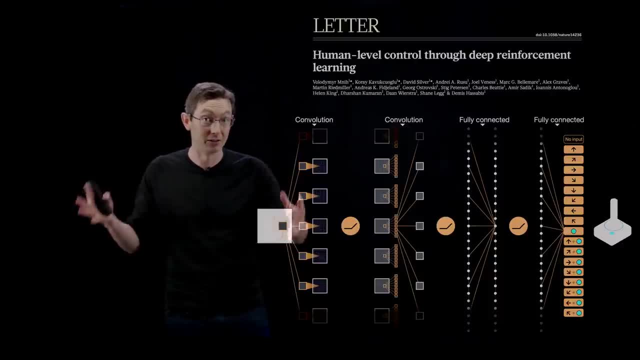 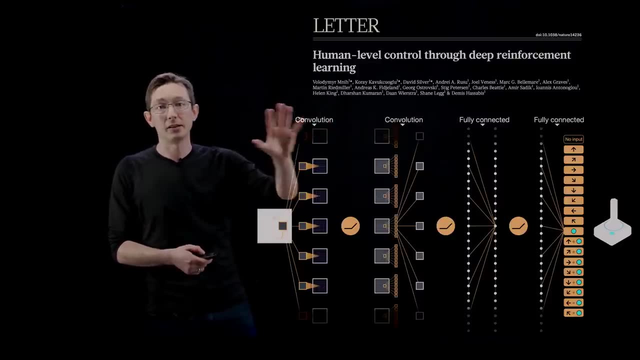 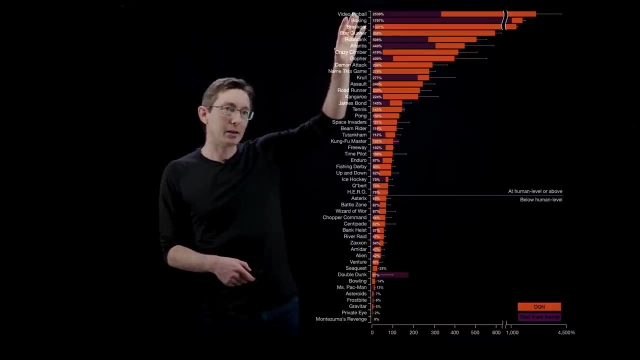 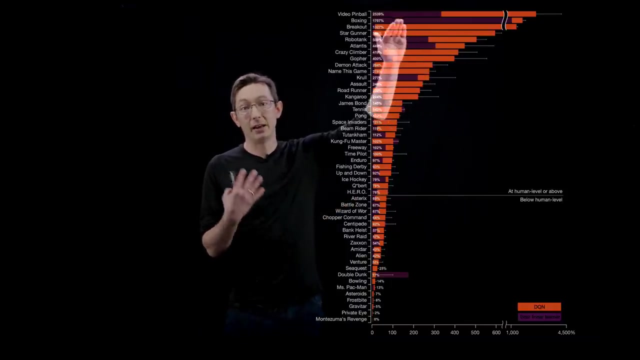 artificial intelligence or an artificial intelligence system that could get good at lots of things, rather than just one very specific task. And since then, billions of dollars have been invested into reinforcement learning in general and deep reinforcement learning by companies, And so in this original paper, these are all of the Atari games that they try out, And this is the level above this they beat. 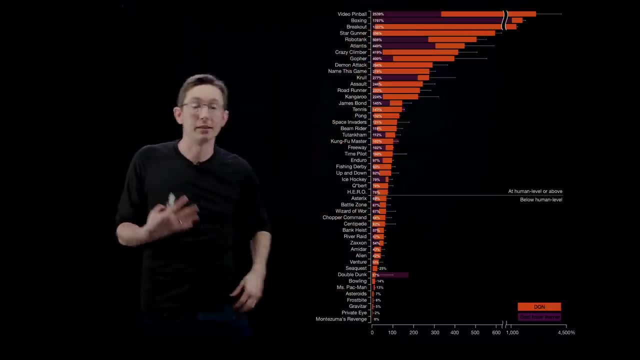 They're at or above human level performance and there's only a few games that they're below human level performance And I actually think it's pretty interesting to look through these and figure out why this deep mind was unable to figure out these games. but it was able to figure out these games. That's kind of an. 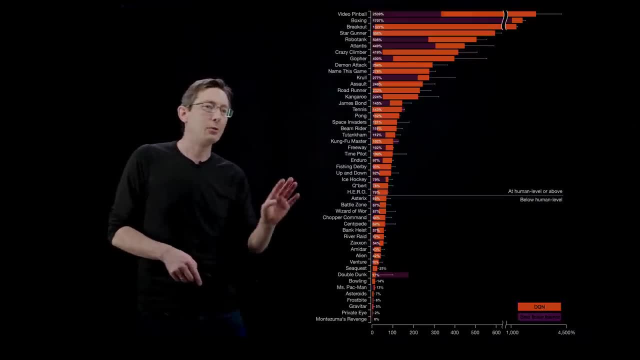 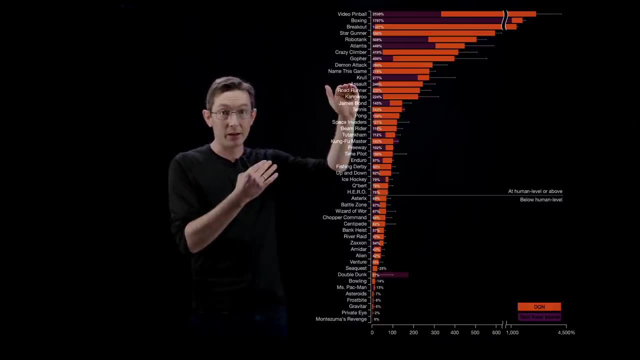 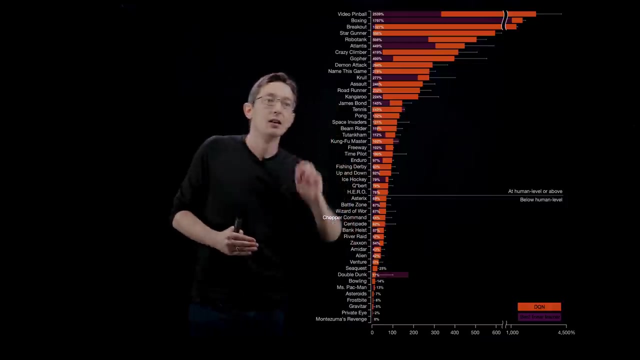 interesting exercise. Actually, I will point out that the algorithm in this paper, you could train it on one of these games and it would get really, really good. But that same learned algorithm, that reinforcement learner, cannot then be used to play another game without completely retraining it. And so it's still a way, you know, a ways away from where we want to be. 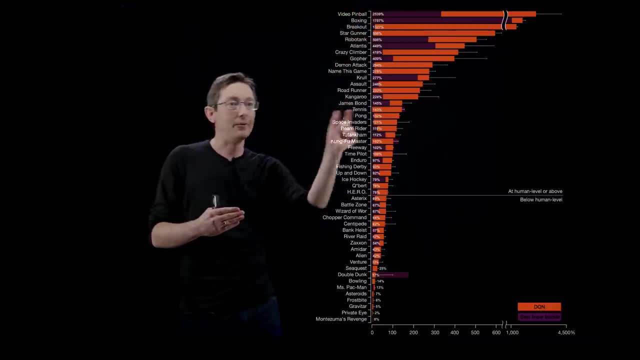 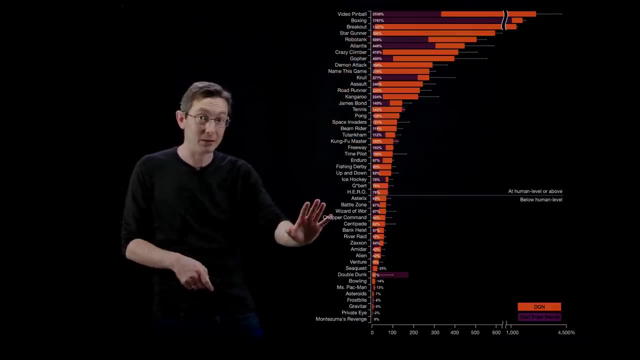 We want to have a learning system that can learn to play all of these games And if it learns one, it can learn how to play the other faster And better, just like a human does. We're still a ways away from that, but tons of people are working on it. It's one of the big, big. 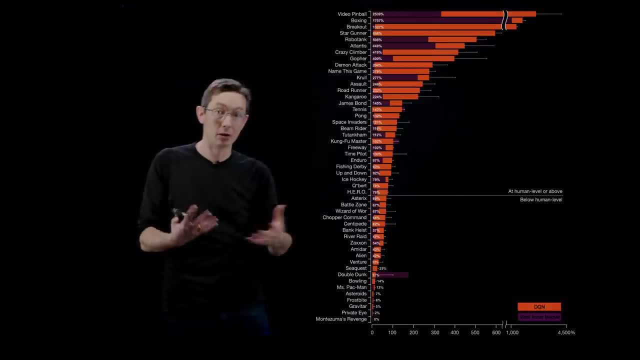 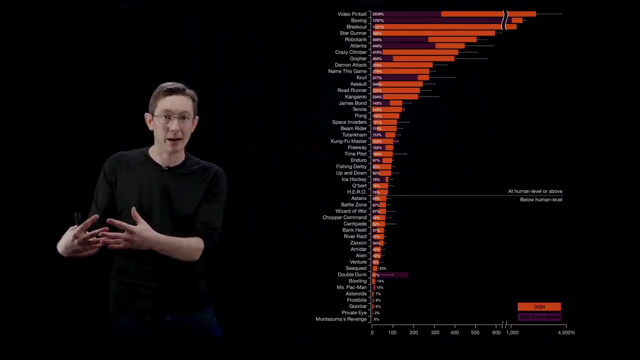 problems in the field is kind of transfer learning and general artificial intelligence using reinforcement learning. So building a learner that can learn lots of things and learn faster from its experience. That's what humans do. You get a kid, you teach him tic-tac-toe. Tic-tac-toe is easy. They learn the rules, They learn how to not lose. 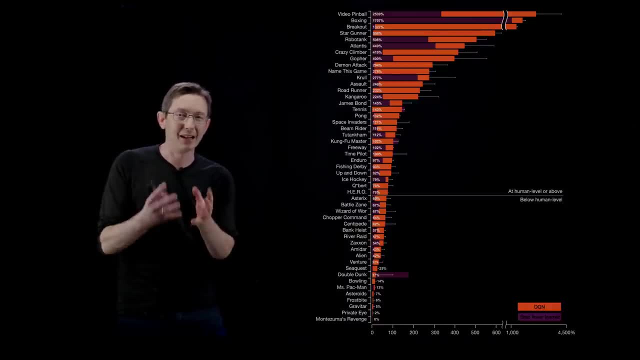 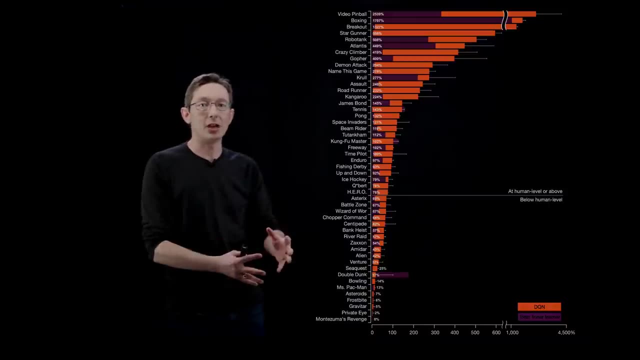 Then you give them checkers. Checkers is a little bit more sophisticated, but they remember everything they learned from tic-tac-toe and they learn checkers faster. Again, they learn how to not lose. Then you give them chess. Chess is a truly open-ended game for most humans. It takes a lifetime to master. 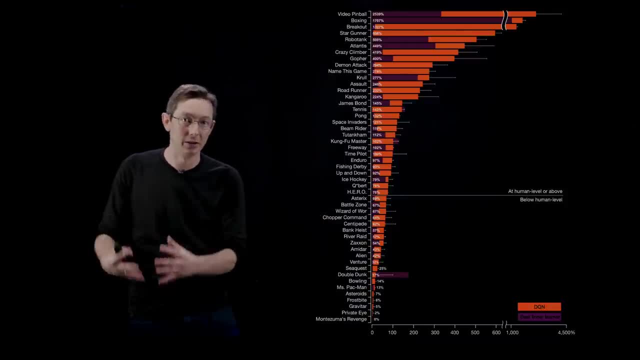 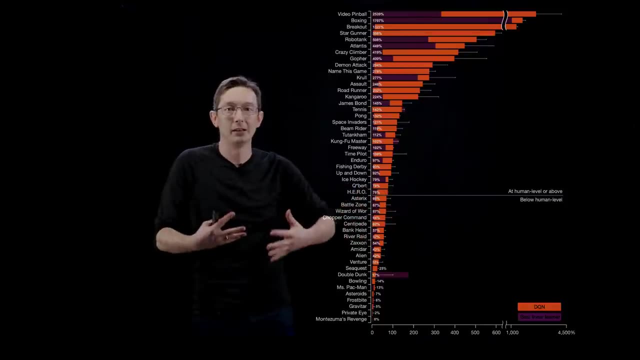 And so, based on what they know from tic-tac-toe and checkers, a child will learn chess. You know they can transfer some of that over and then they go into the real world and they learn lots of other skills, and those problem-solving skills transfer over. That's what we 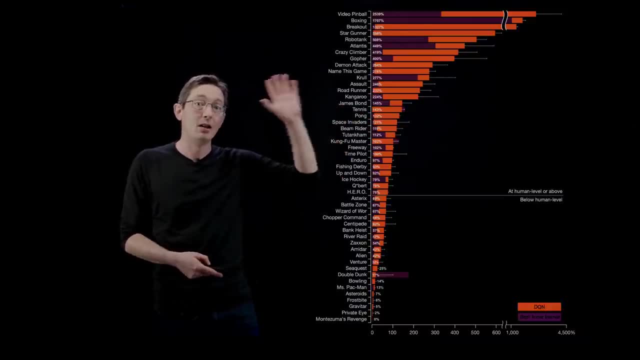 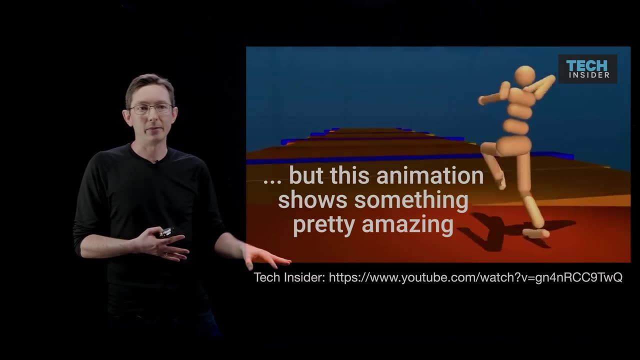 eventually want with computers. We're not there yet, but this was a big step and it got everybody really excited and still does Good. This is another video I love. This is from the Tech Insider, showing you know a lot of these reinforcement learning algorithms are used to train. 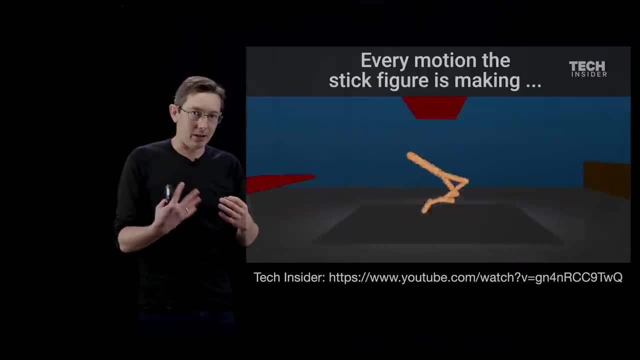 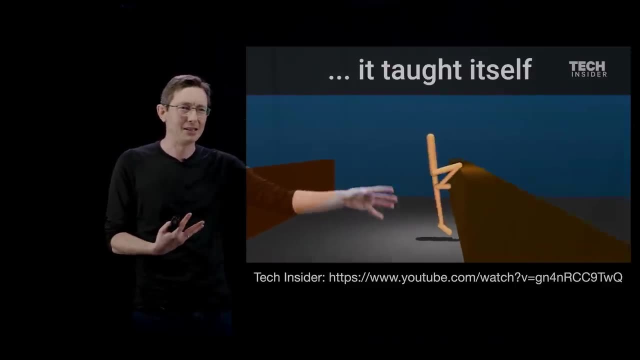 to train the agent how to walk or run or leap or swim or fly in an artificial environment, And that's pretty amazing. I mean this is a very complex, hard thing to do. We take it for granted: Our bodies are built to move very efficiently. 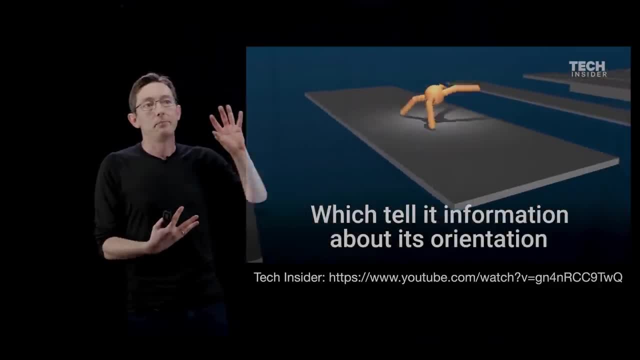 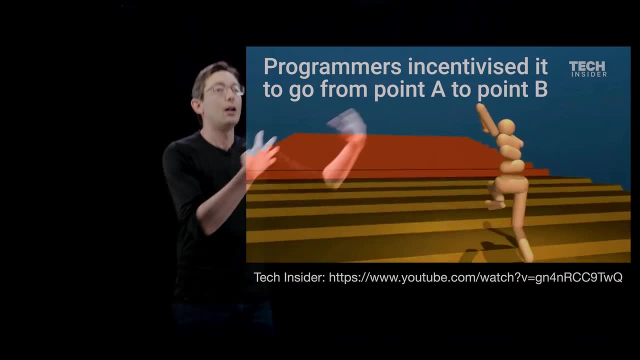 and in agile and accurate ways. But this is actually very challenging to do, And so the fact that these algorithms in a virtual environment can learn how to run and walk and fly and swim is really promising for robotic technology. So we eventually want to learn how to do this. 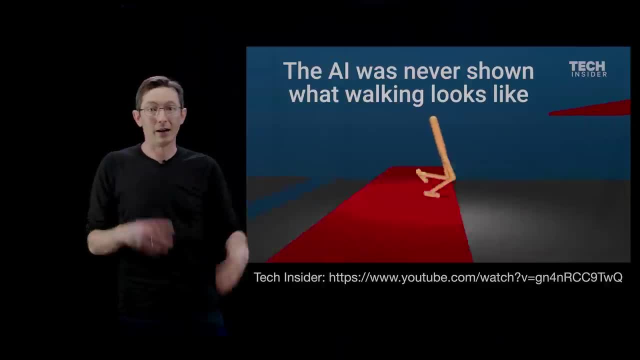 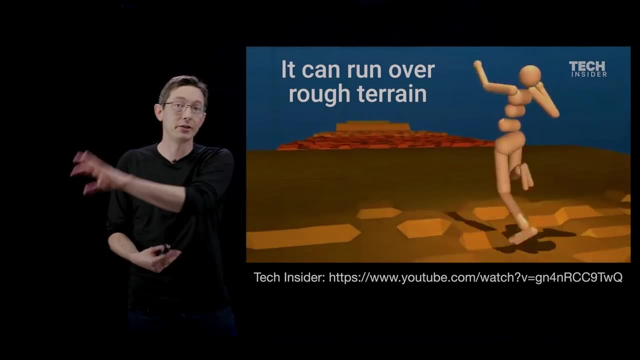 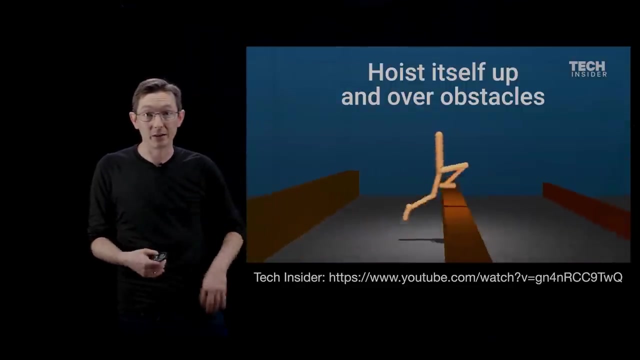 in robotic systems and make our robotic agents more independent and more agile, And that's actually really hard. That step from the artificial world to the real world is challenging. So, for example, to my knowledge, Boston Dynamics does not use a tonne of reinforcement learning. 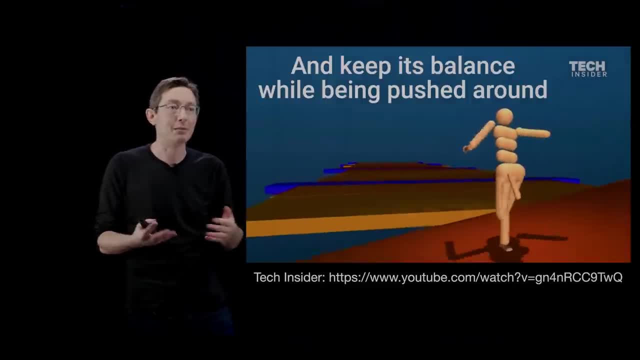 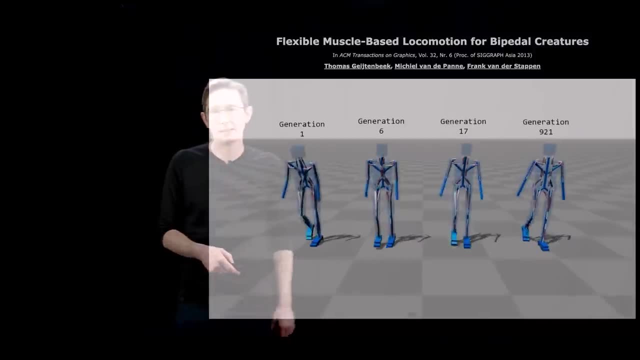 They use a lot of physics-based modelling and kind of by-hand controls. Maybe they're getting into reinforcement learning, but there's a long way to go to do this in the real world. Still quite impressive, And this is a video I love. So this is training bipedal walkers. 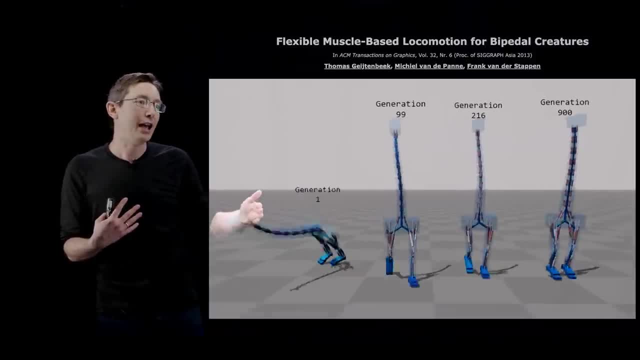 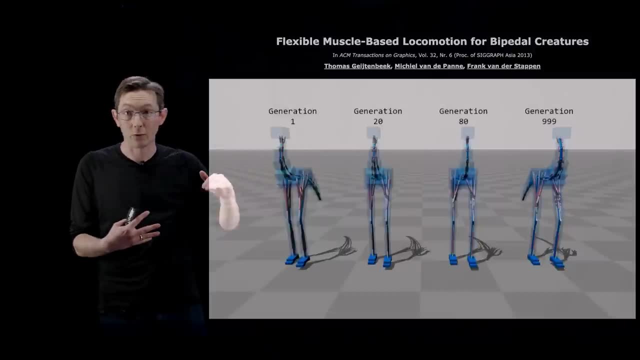 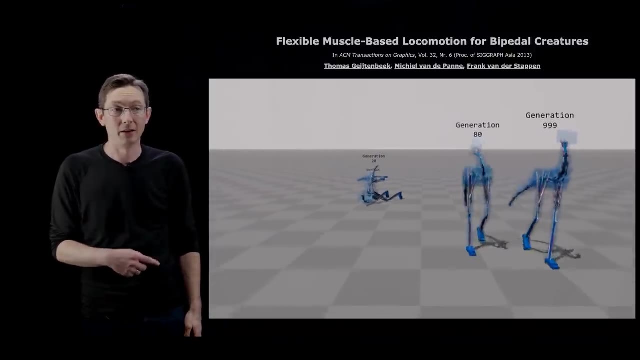 essentially generation after generation of reinforcement learner And eventually the agent can learn kind of the physics and learn the right control policy, in this case to walk forward stably and, you know, keep its neck straight and keep its legs straight. And I think this is just a really cool video and a nice demonstration, I'll point out. 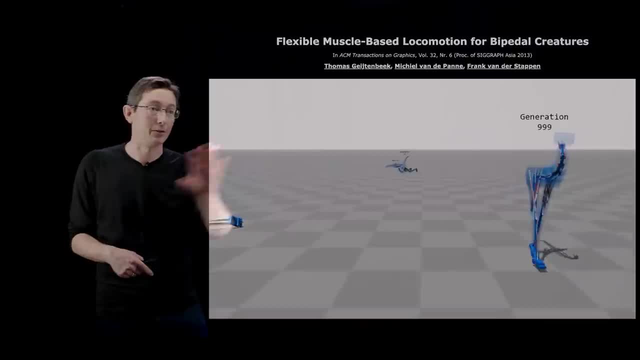 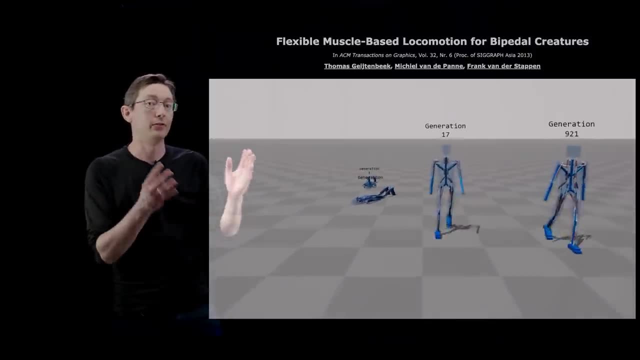 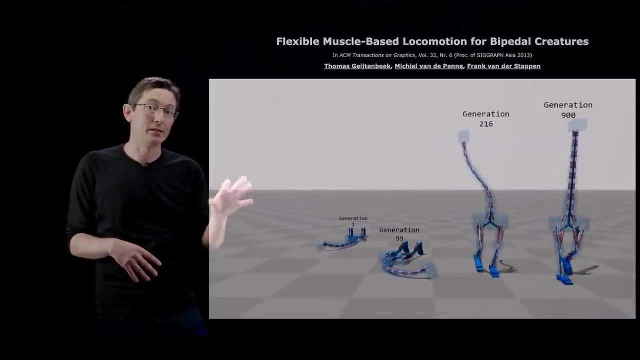 there's some great resources. Other resources on YouTube you should check out for reinforcement learning. I learned about this in Two Minute Papers, which is a great channel. I love, love, love learning about things in Two Minute Papers. There's also Archive Insights has a great series. 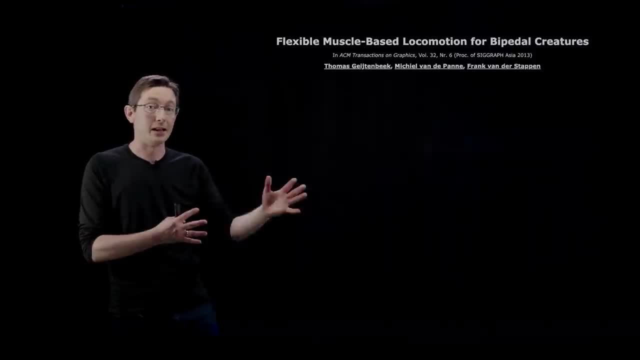 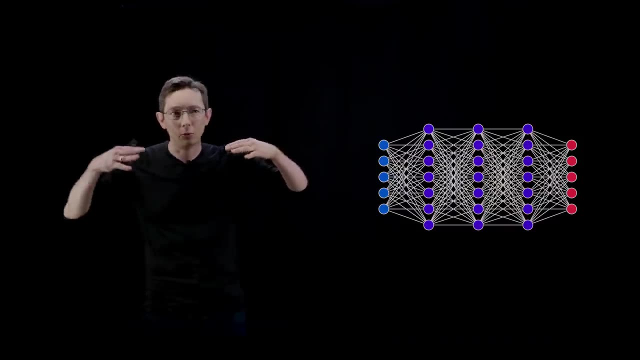 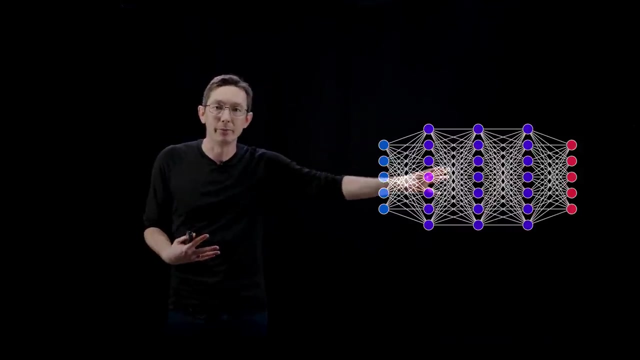 on reinforcement learning, And Brian Douglas has a nice kind of reinforcement learning for control video. I believe it's on MathWorks. Okay, good, So really impressive performance just in the last 10 years because of these huge advances in the representational power of neural networks. These 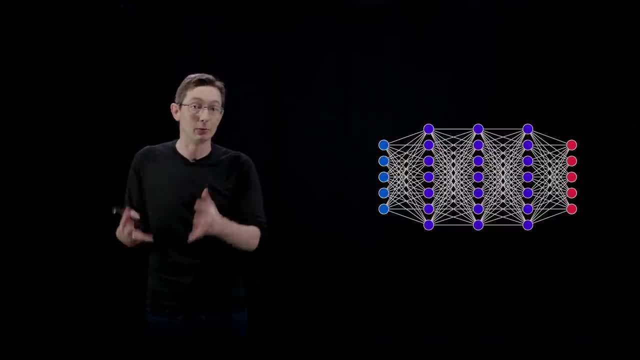 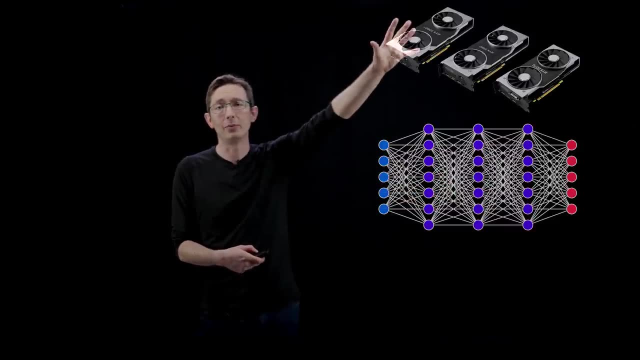 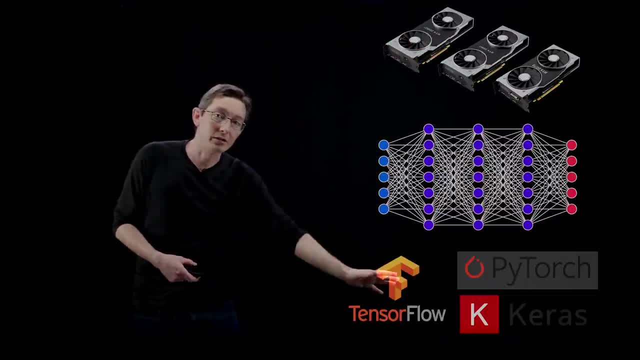 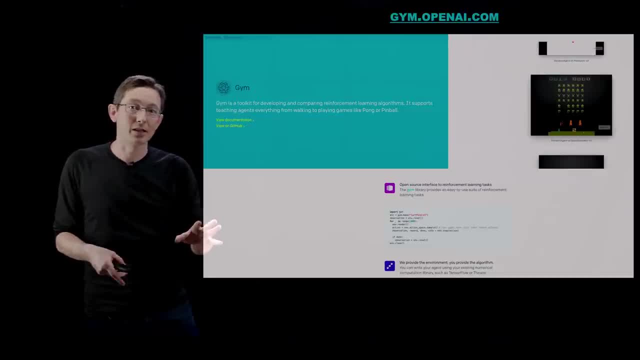 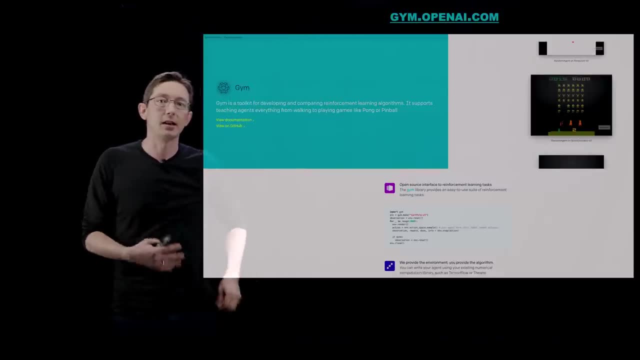 representations, And so if you have any interest at all in modern reinforcement learning, you have to check out OpenAI Gym. This is a wonderful open source kind of development framework where you can try out your new reinforcement learning algorithm on all of these different systems, both Atari games. 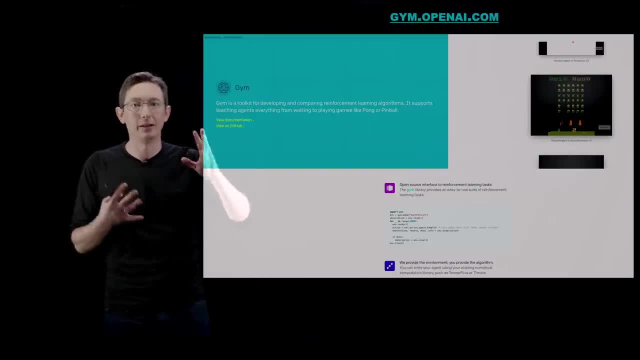 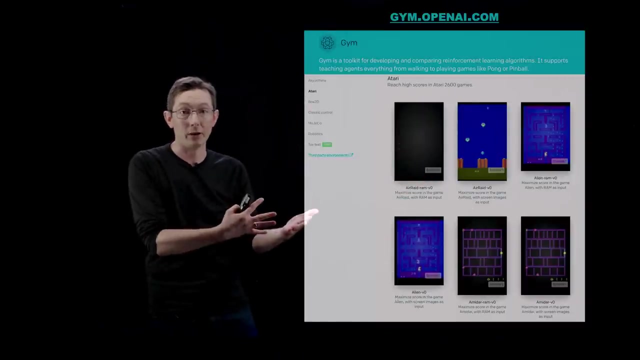 simulated, you know, running and Pendula and really cool physical systems that are hard to control, that are non-linear. You can get started really quickly and easily in the OpenAI Gym And this is one of the big reasons things are taking off so fast is because there are these amazing open resources for people to kind of try things out quickly and rapidly, prototype And again you can try out all of these Atari games and see if you can build a reinforcement learner that can learn multiple Atari games with the same architecture. That would be pretty incredible. 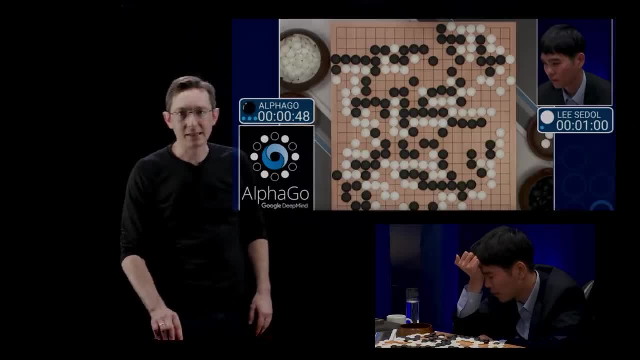 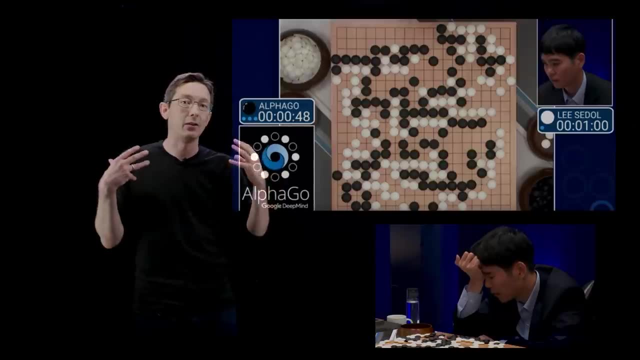 Thank you. Okay, I also want to point out these things are getting pretty impressive. So almost everybody's heard of AlphaGo and how AlphaGo beat the human best Go player in the world, Lee Sedol from South Korea. The best Go player in the world- was defeated by AlphaGo. This was a deep reinforcement learning algorithm developed at Google DeepMind with the sole purpose of 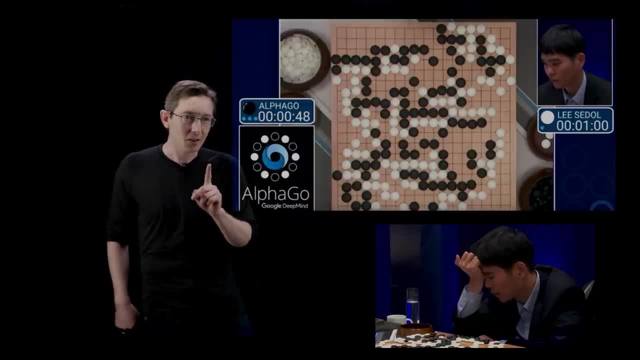 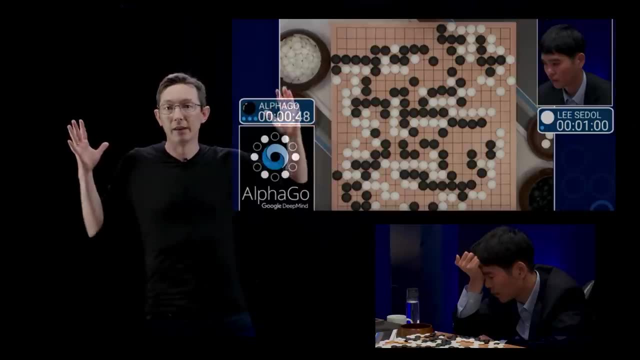 learning how to play Go Okay, And so I want to point out that. so reinforcement learning is really good at learning the rules of the game and how to win the game when it's very constrained and when it has all the time in the world to try millions or billions of different Go games. So it's playing essentially with itself, getting better and better and better. Lee Sedol is a human and he has a life, And although he spends much of his time in the Go world, he has a 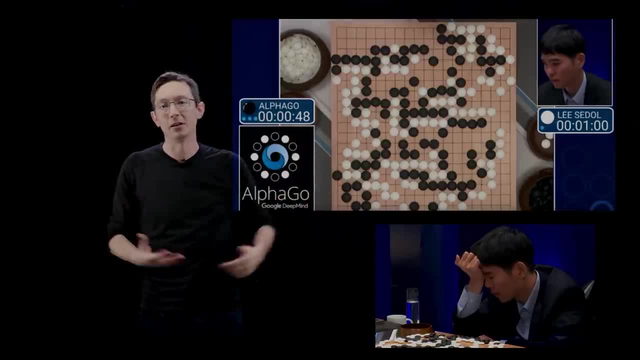 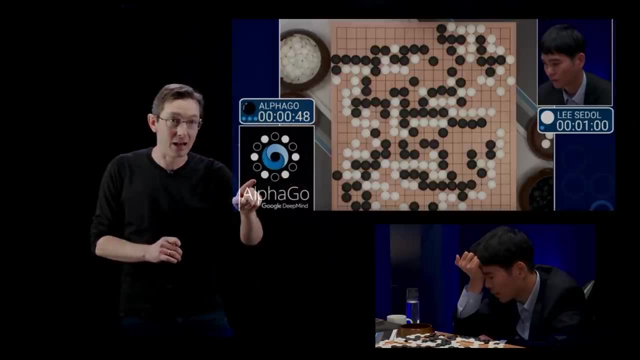 much, much richer, broader world And he can go home and he can go for a walk and he can enjoy a sunset, And so I do want to point out that and he can learn from AlphaGo and come back and be better the next time. And I think that's really also quite impressive is that the human masters learned from DeepMind and actually got better once they played up to their competition. I think that's really cool. But anyway, this AlphaGo learning system, 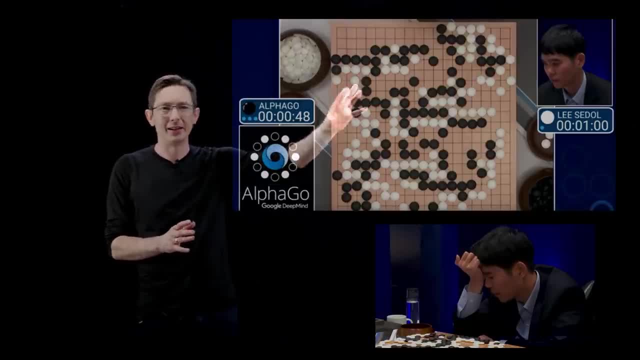 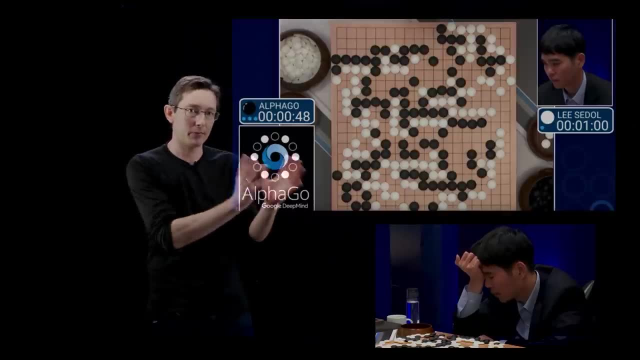 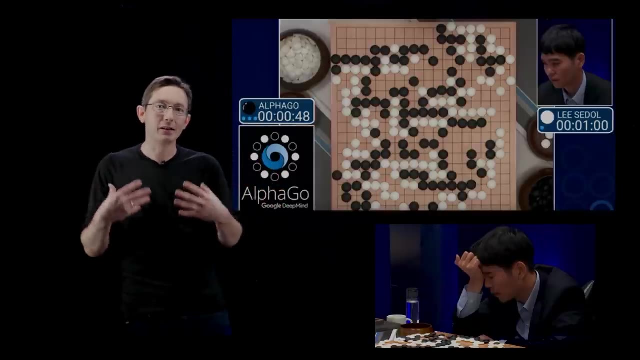 I think is really interesting. This deserves a whole set of videos just to dive in. I think there's a documentary on this. It's really interesting, So you should check it out. The original AlphaGo algorithm was based on a convolutional neural network, a CNN, and it had lots of reward shaping from humans. So expert humans guided the reward structure for this AlphaGo learner. So it didn't have to wait until the end of the game to figure out if it won or lost, because that would take forever. 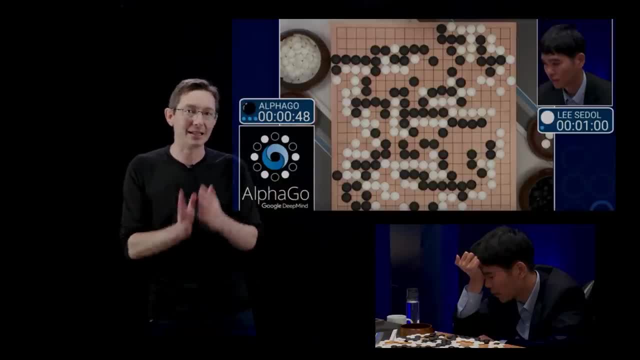 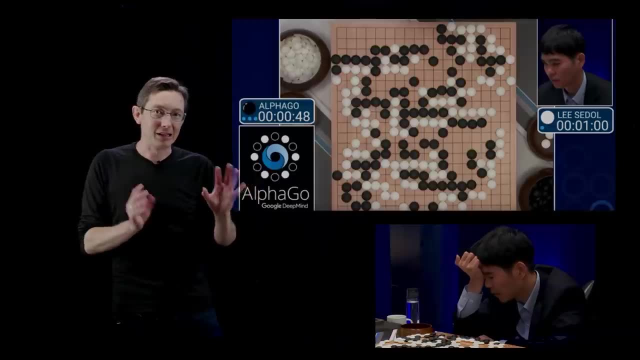 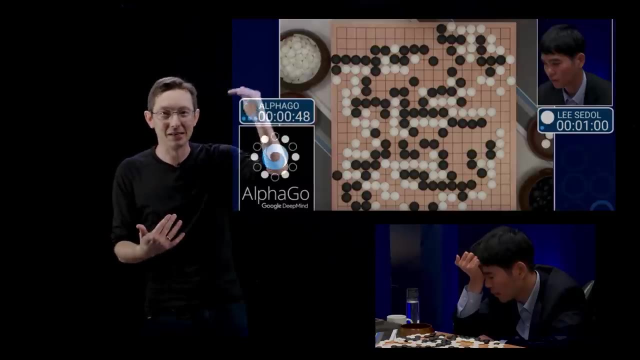 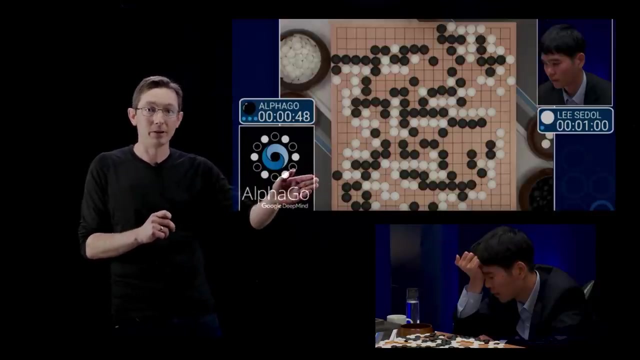 Instead, humans, using reward shaping, helped it to get intermediate rewards to help it to learn faster and give it a denser reward structure. Now, that's tricky because if a human guides the learning, that almost caps out how good it can possibly be, because it's fundamentally relying on human knowledge. So the next generation, AlphaGo Zero, which came a couple of years later, was even better and much more impressive. It didn't use any human features. 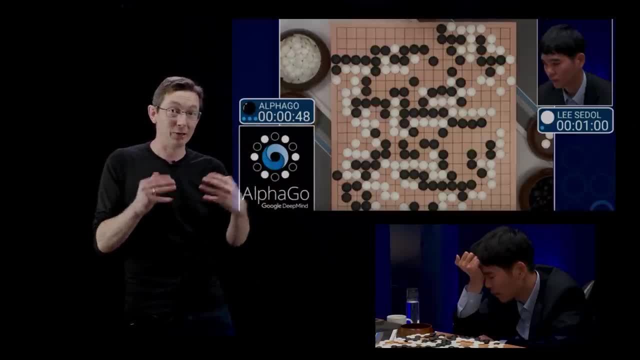 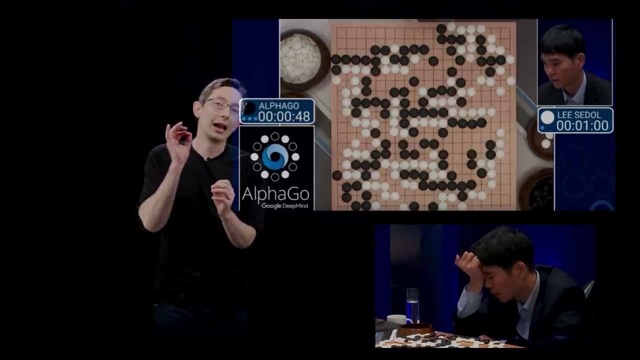 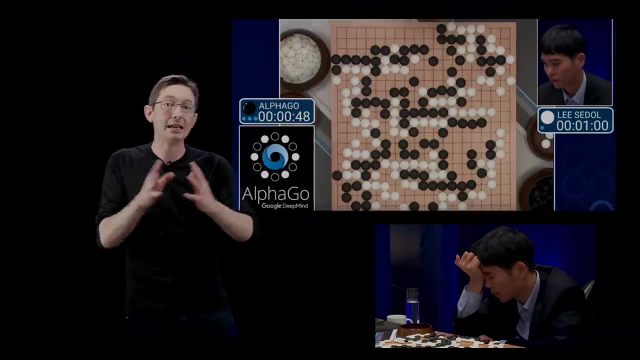 There's no reward shaping It only learned using self-play. It just played itself until it became so powerful that it could beat everyone in the world, including the original one, And it was based on a residual network architecture that had these jump connections and are easier to train with back propagation. So really cool advances, And that actually was one of the major advances that showed that ResNet was definitely a good idea. 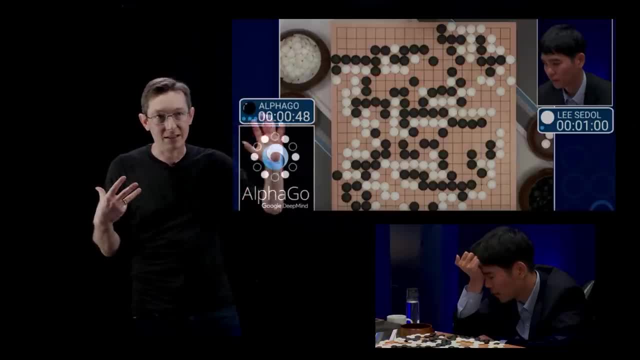 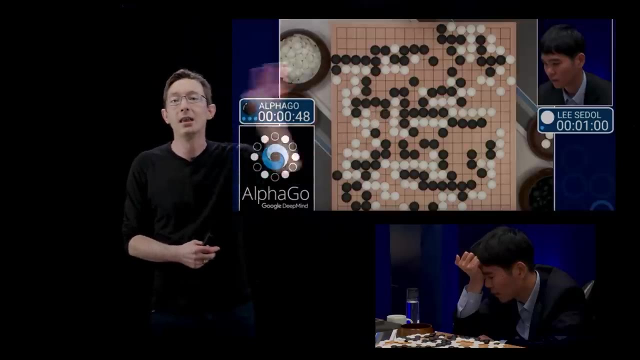 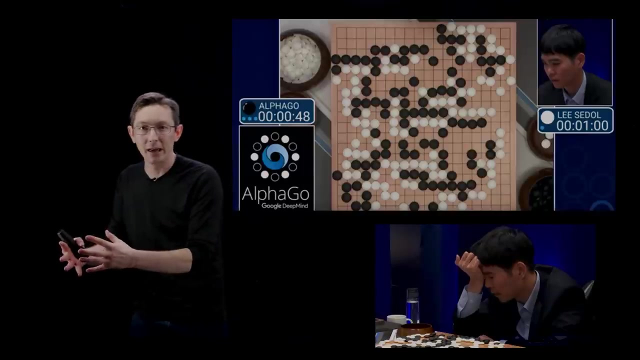 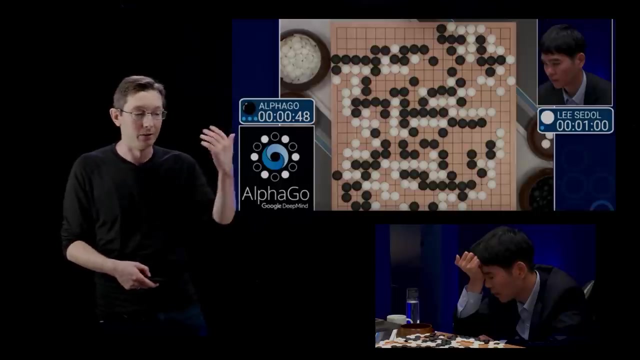 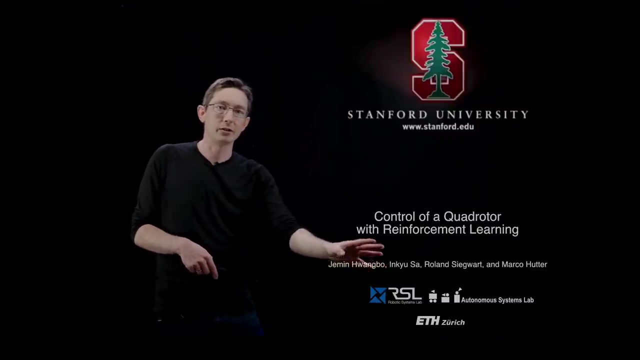 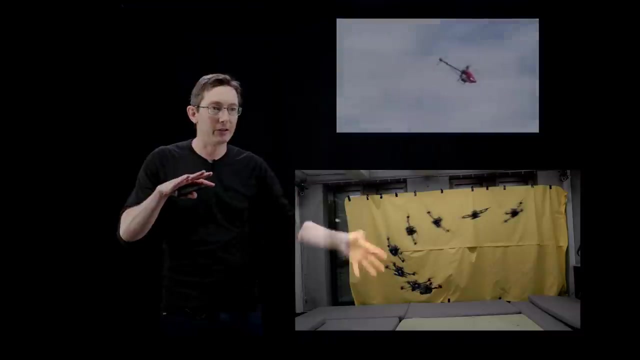 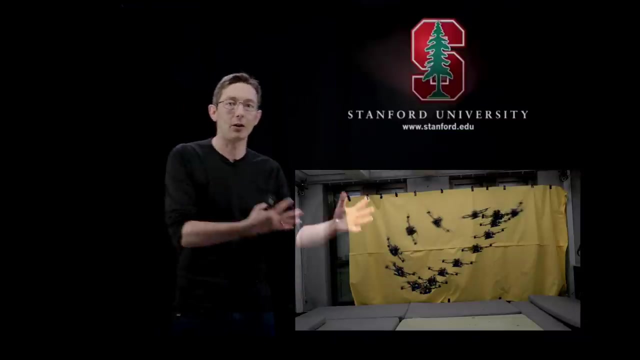 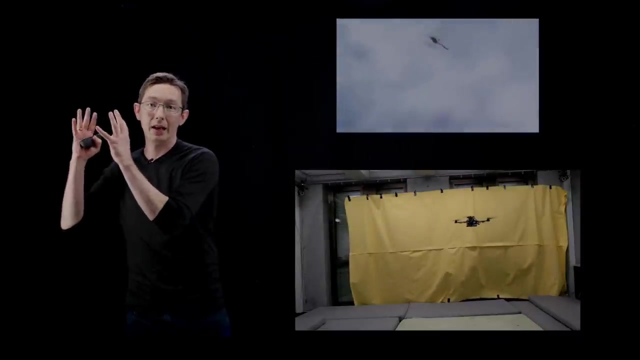 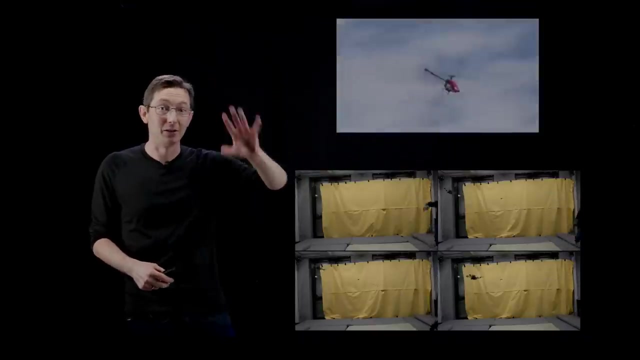 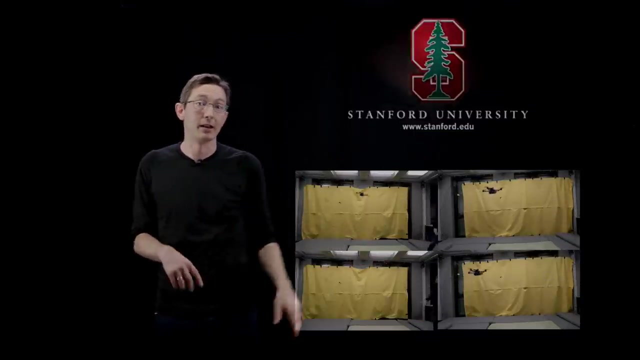 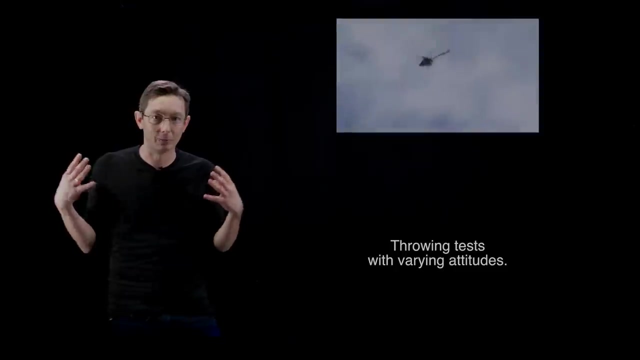 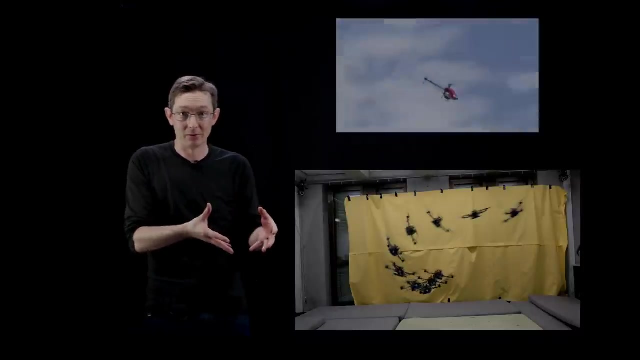 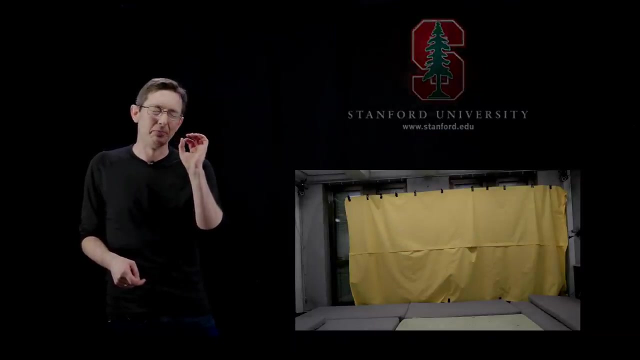 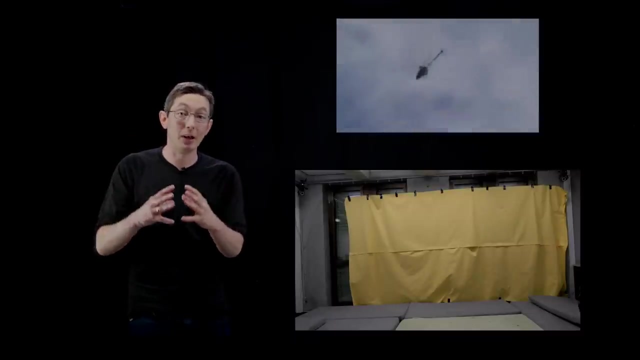 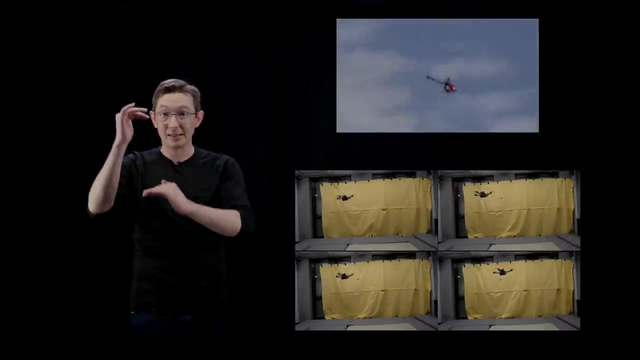 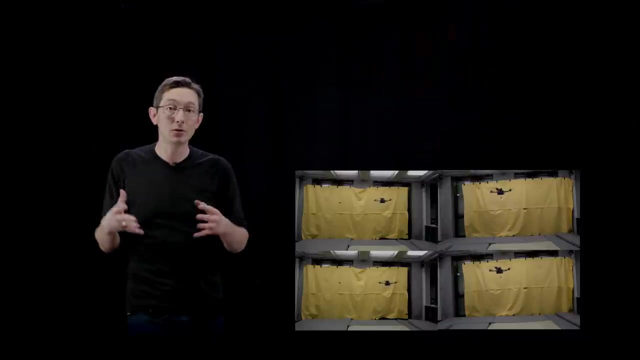 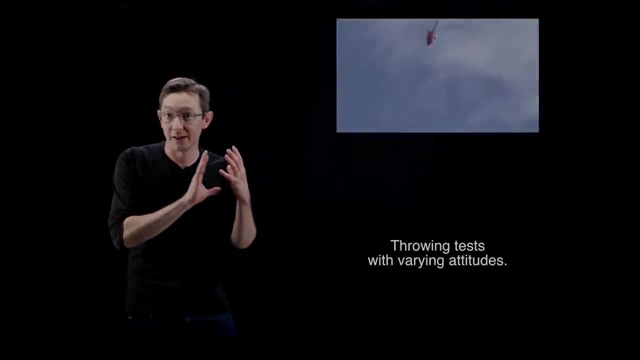 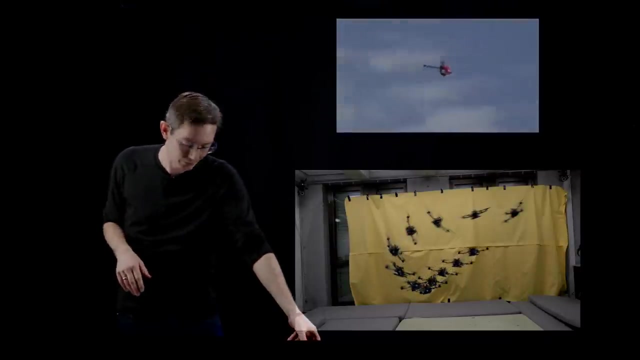 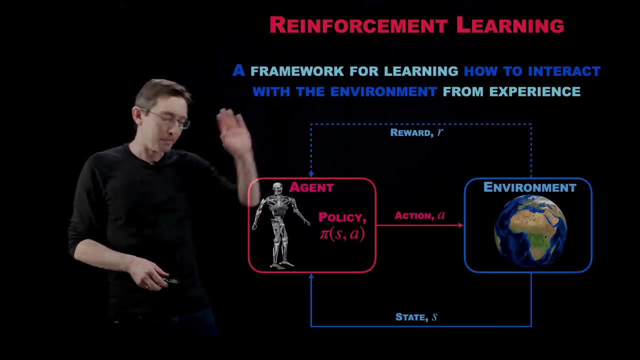 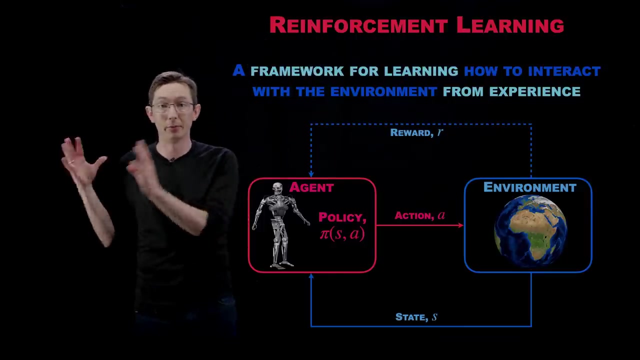 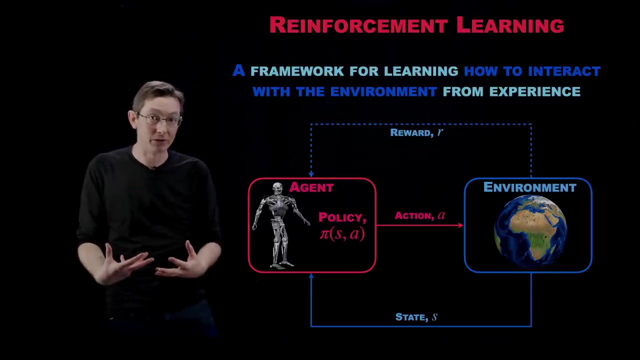